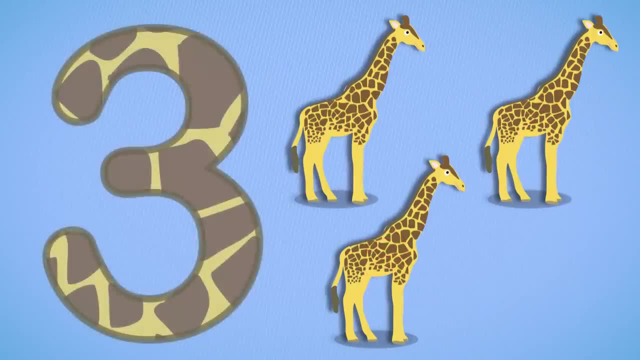 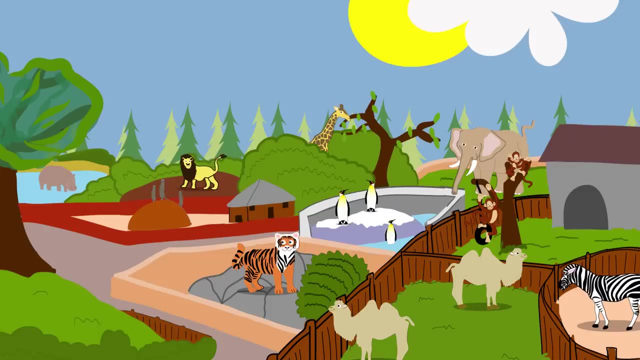 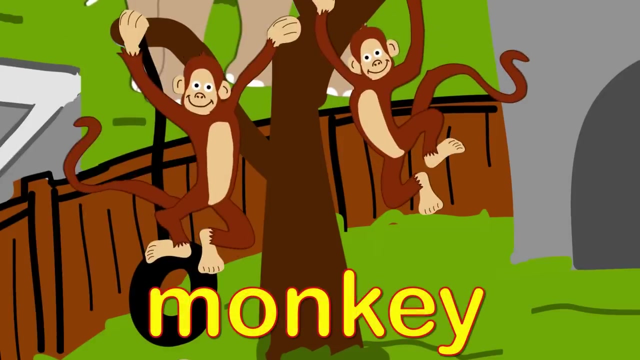 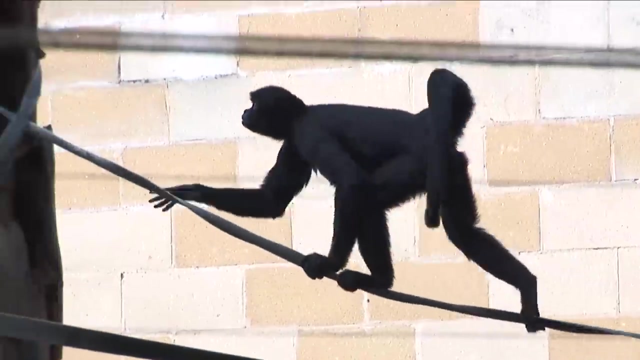 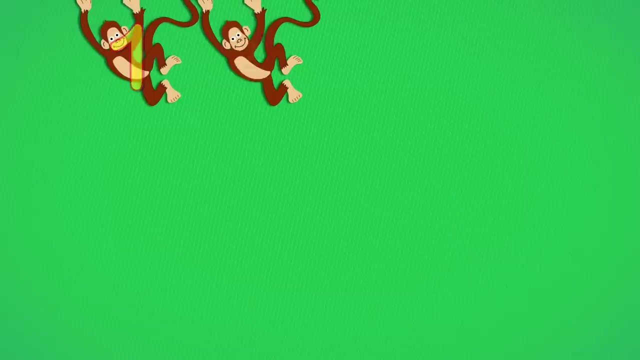 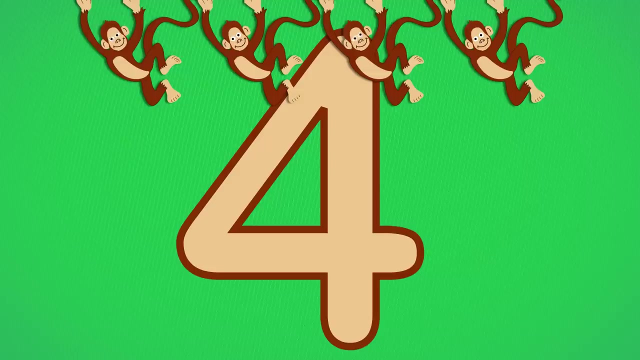 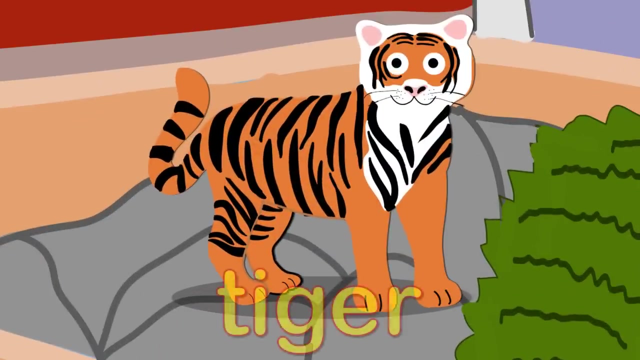 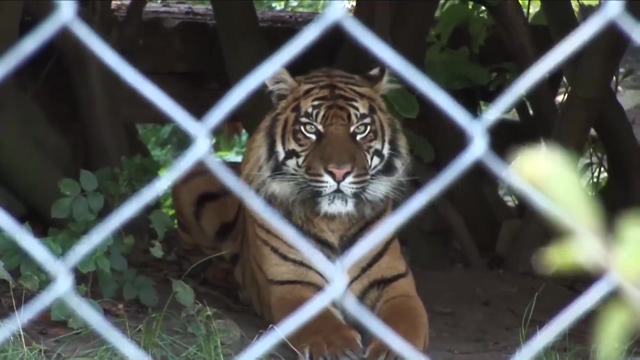 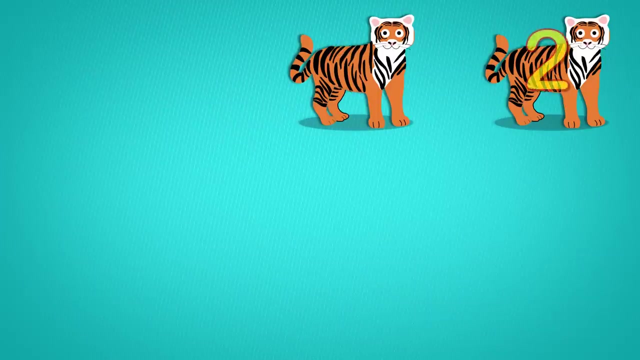 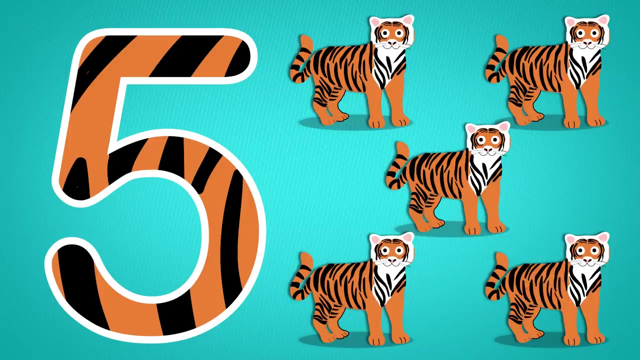 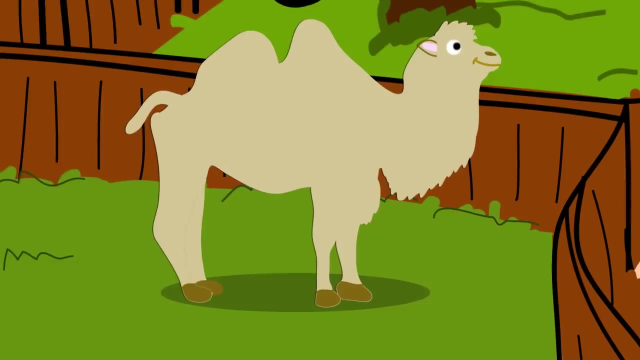 One, two, three, Three giraffes- Hello cheeky monkeys. One, two, three, four, FOUR MONKEYS, Hello Orange Tiger. One, two, three, four, five, FIVE TIGERS- Hello Orange Tiger. 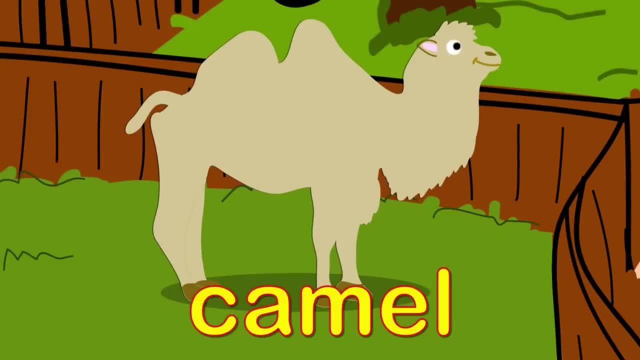 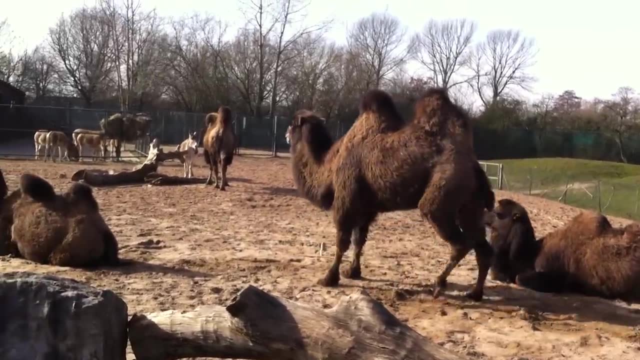 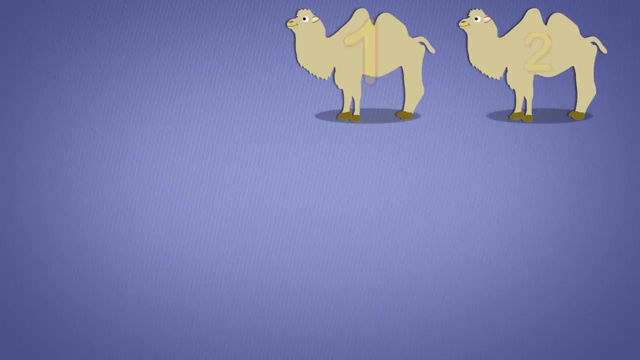 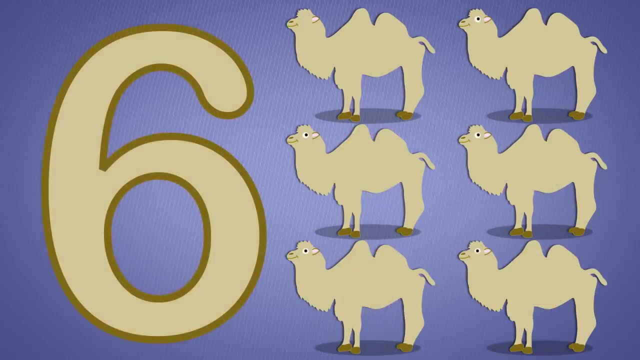 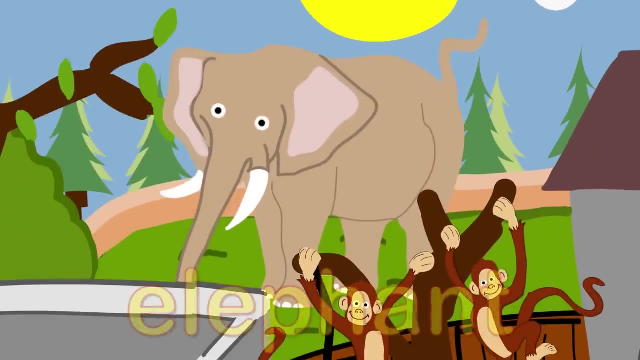 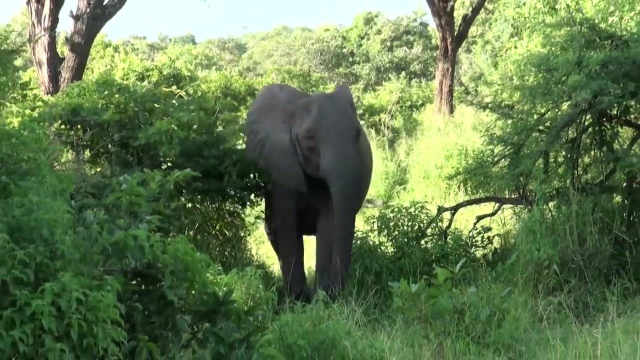 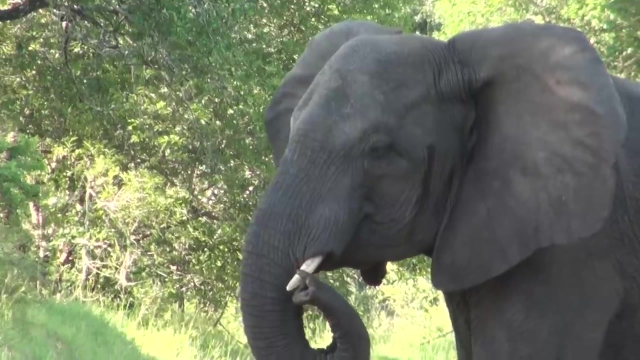 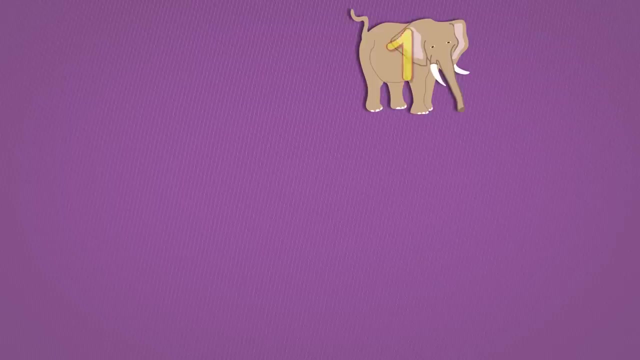 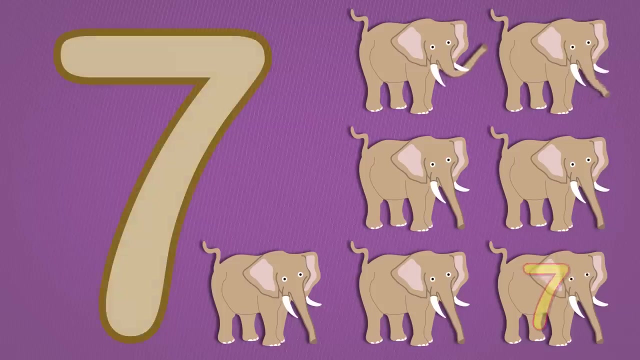 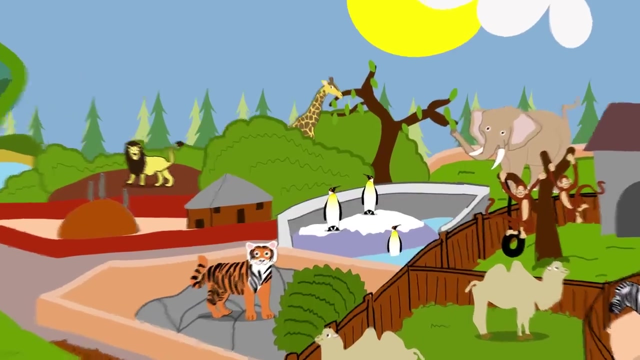 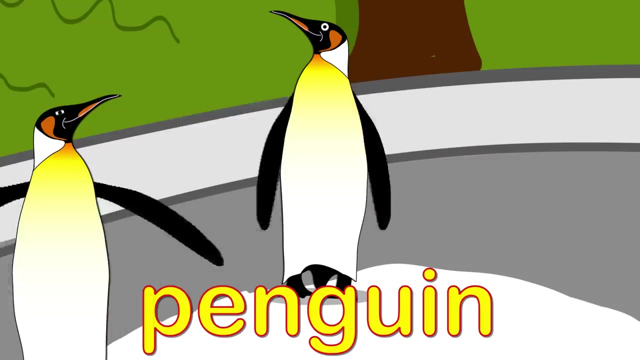 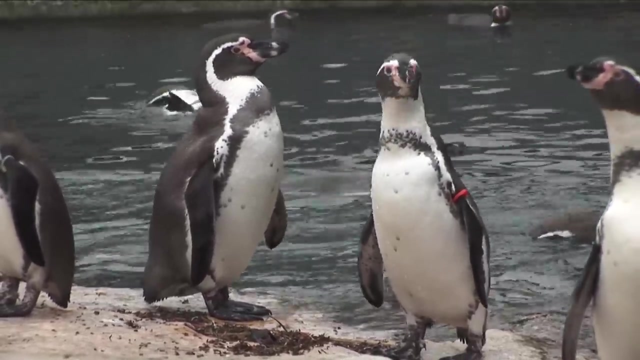 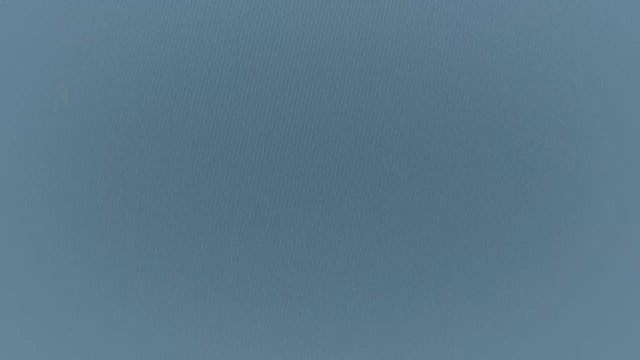 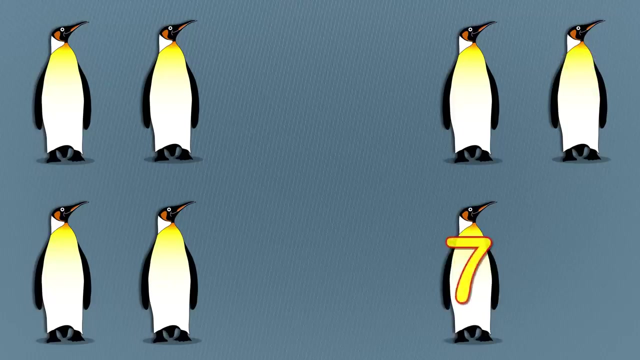 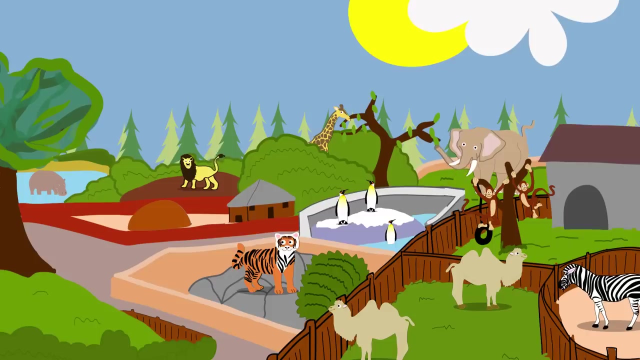 Hello Humpy Camel. One, two, three, four, five, SIX CAMELS. Hello big elephant. One, two, three, four, five, six, seven, seven elephants. Hello pretty penguin. Hello pretty penguin. Hello hungry hippo. 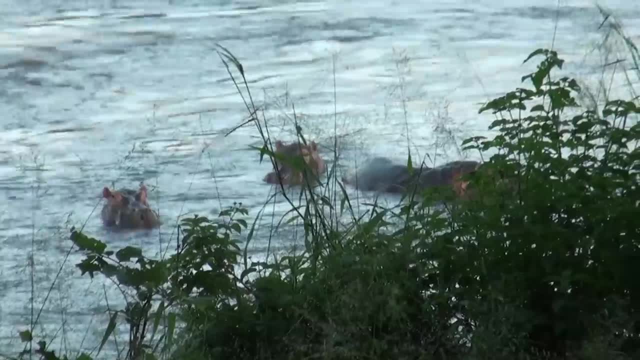 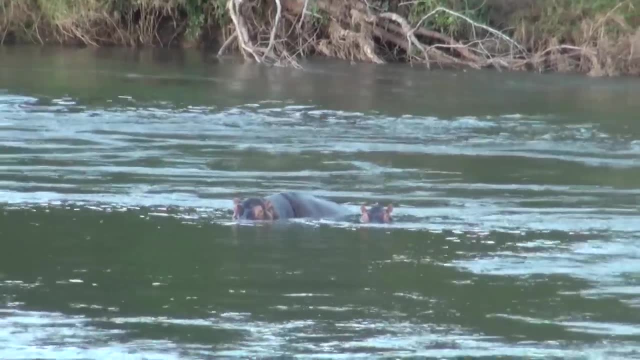 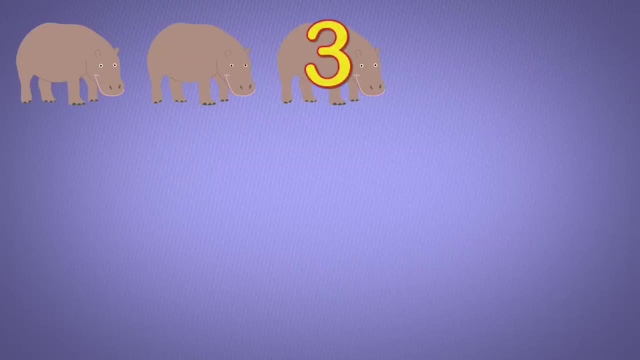 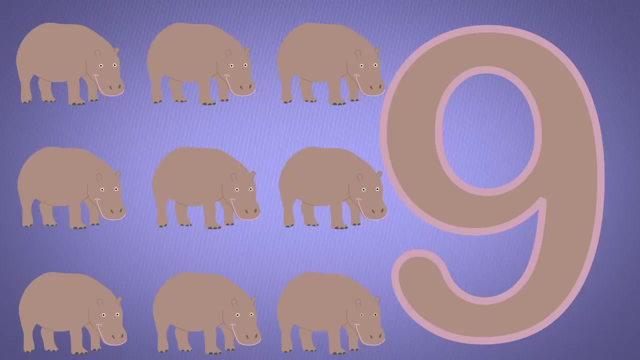 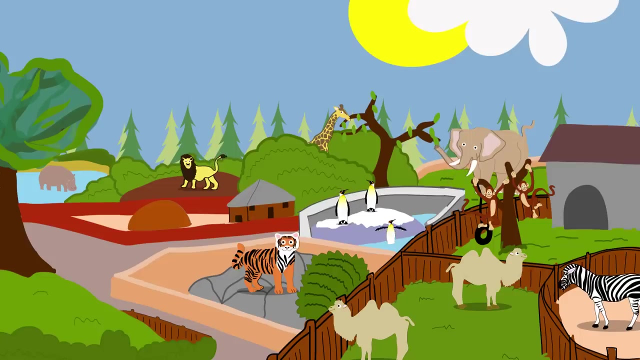 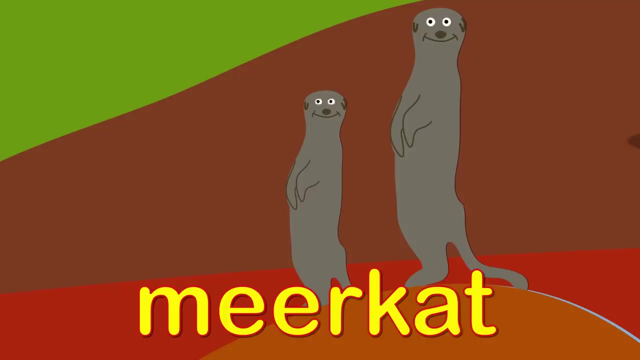 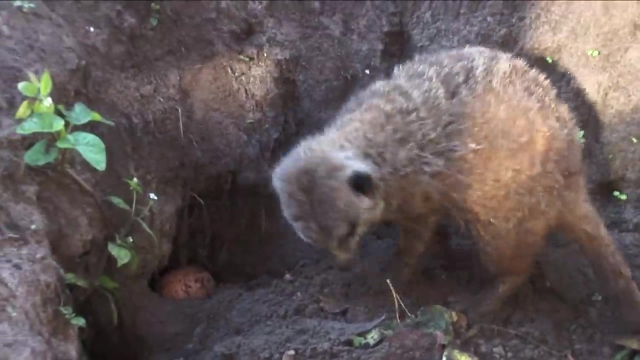 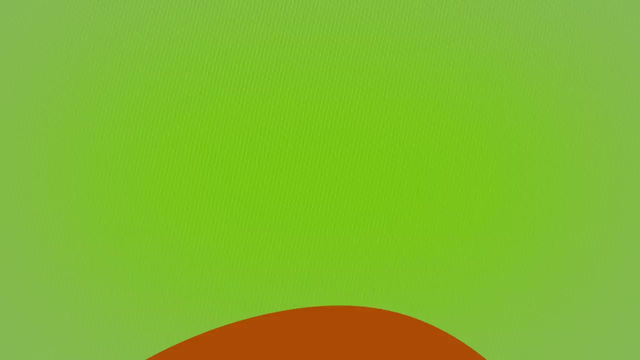 One, two, three, four, five, six, seven, eight, nine, nine hippos. Hello nosy meerkat. One, two, three, four, five, six, seven, eight, nine hippos. Seven, eight, nine, ten, ten meerkats. 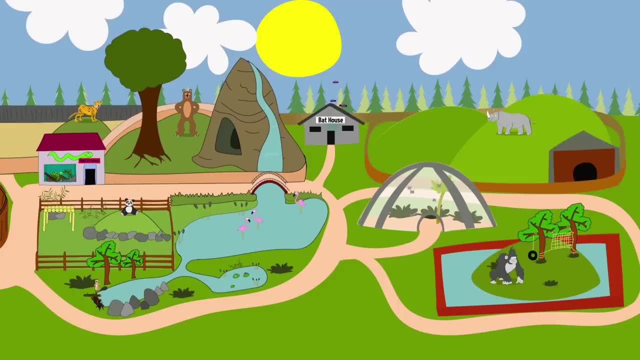 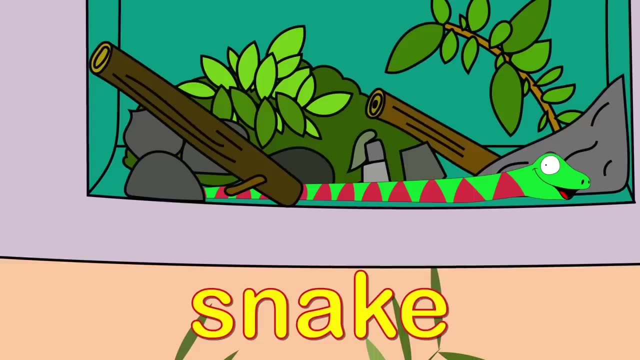 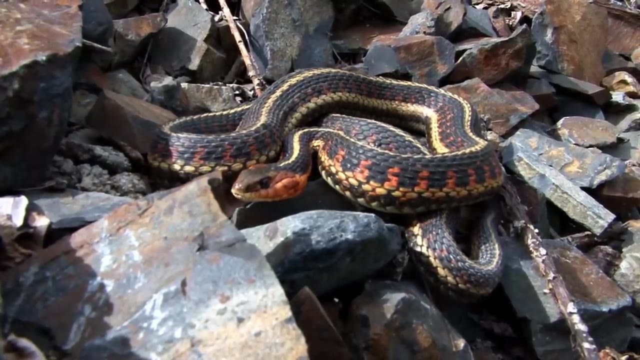 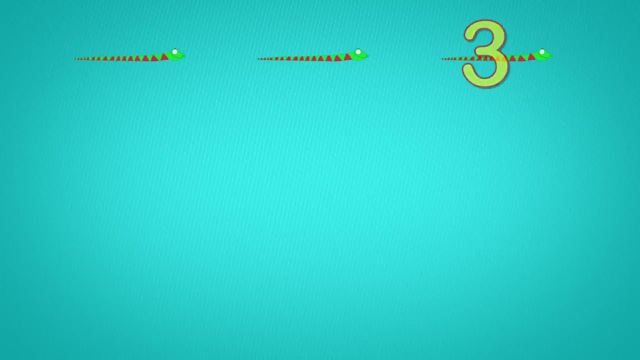 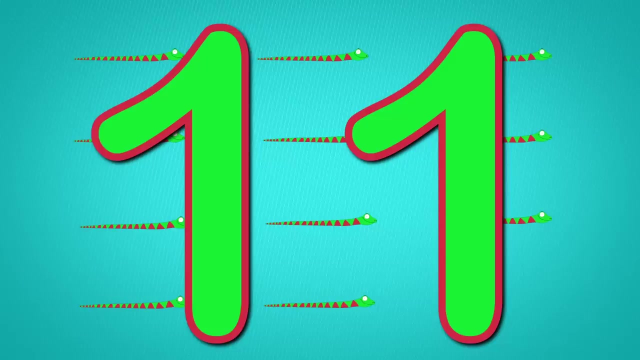 Hello slithery snake. I hope you like your new home. One, two, three, four, five, six, seven, eight nine hippos. One, two, three, four, five, six, seven, eight, nine, ten eleven. 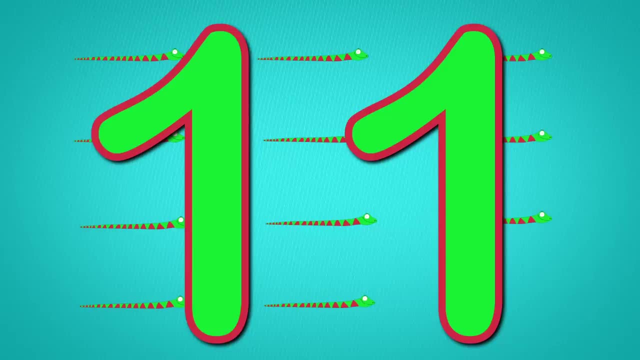 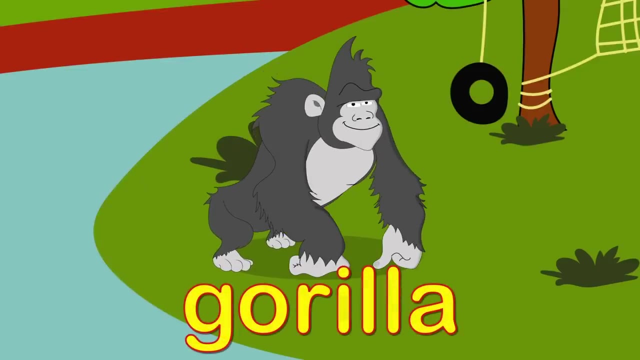 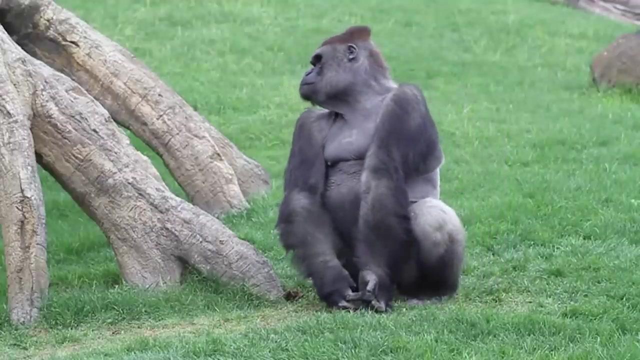 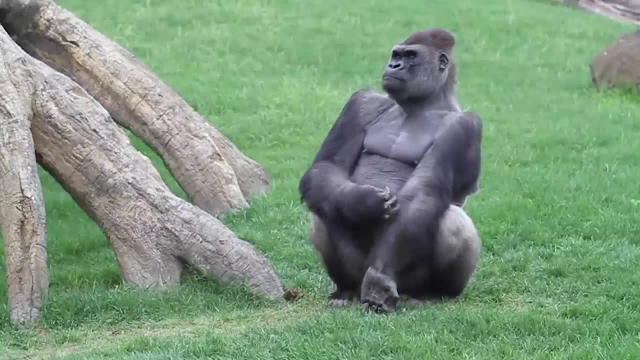 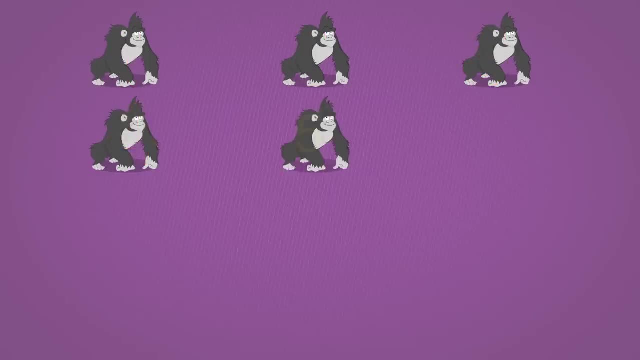 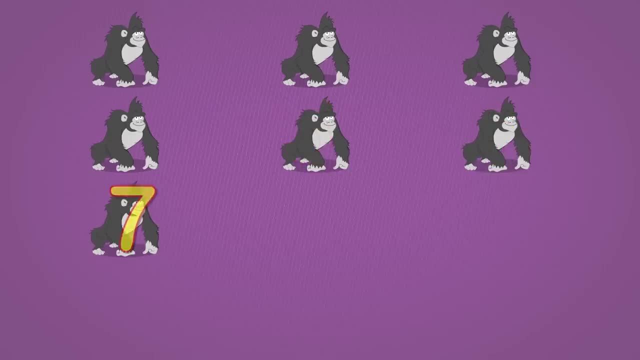 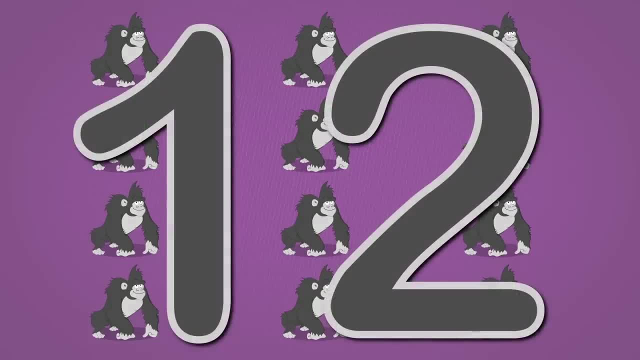 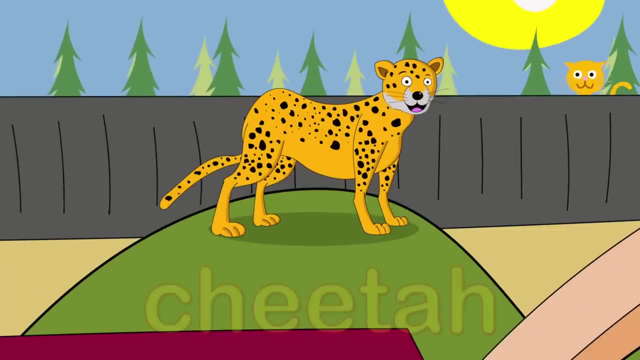 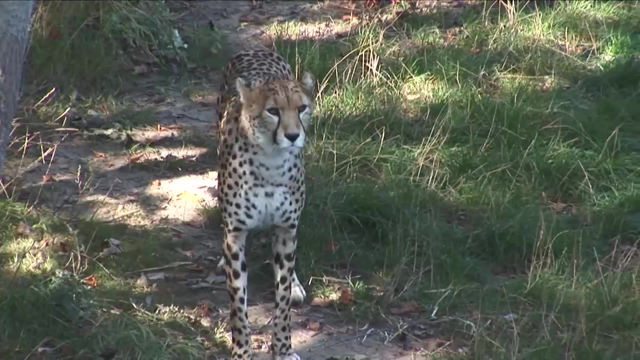 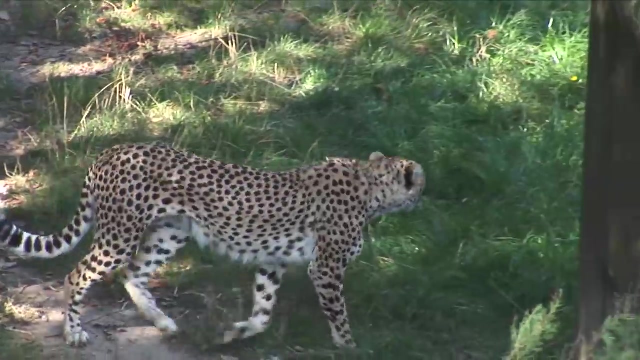 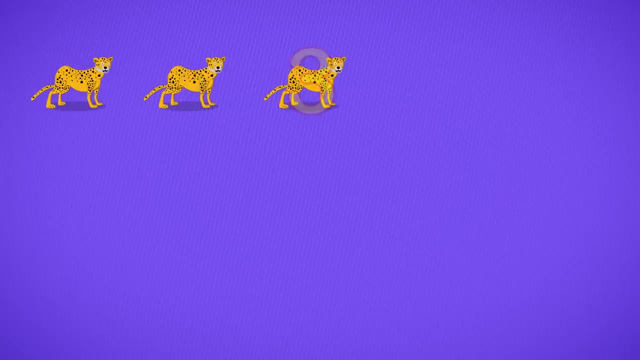 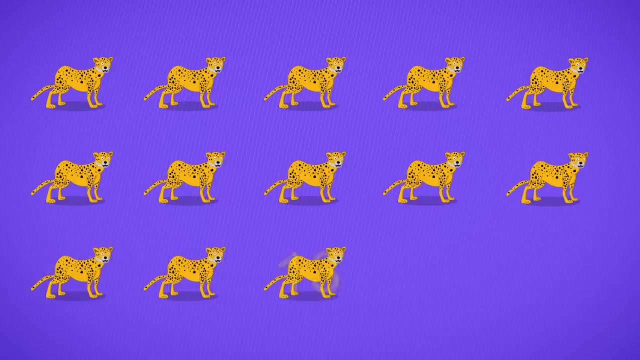 Well hello, Mr Gorilla. Well hello, Mr Gorilla. Well hello, Mr Gorilla gorillas. Who's next? Oh, speedy cheetah, I love your spotty fur. One, two, three, four, five, six, seven, eight, nine, ten, eleven, twelve, thirteen. 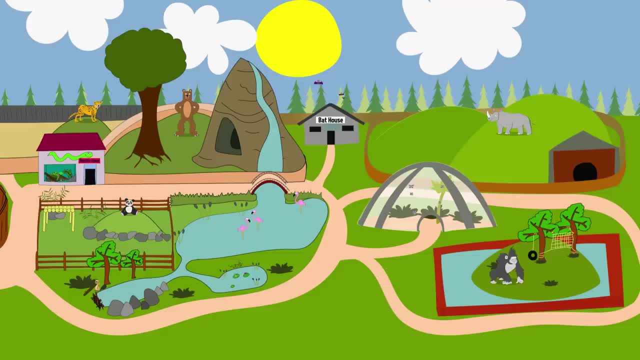 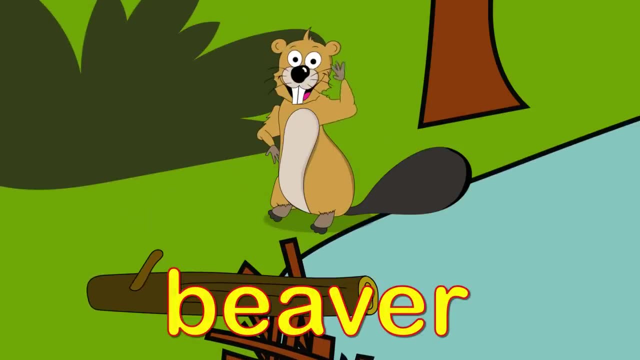 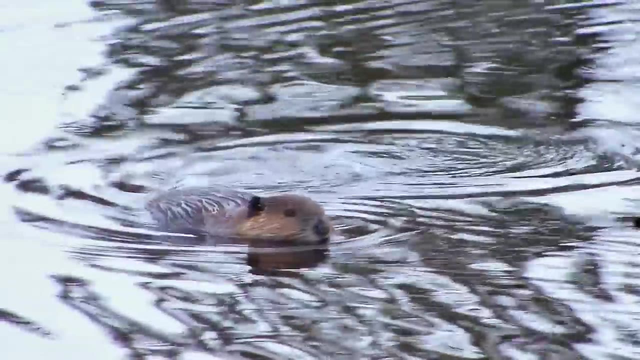 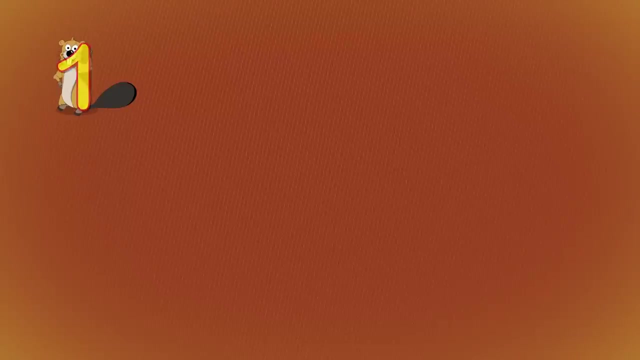 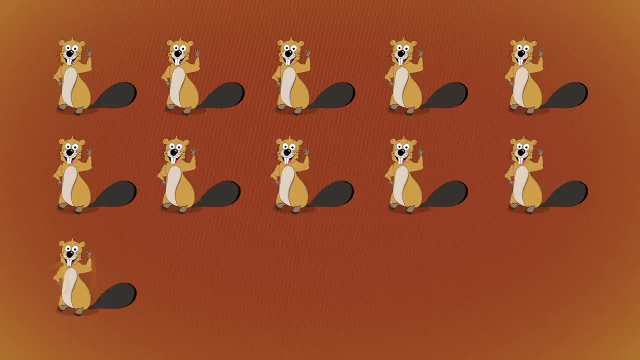 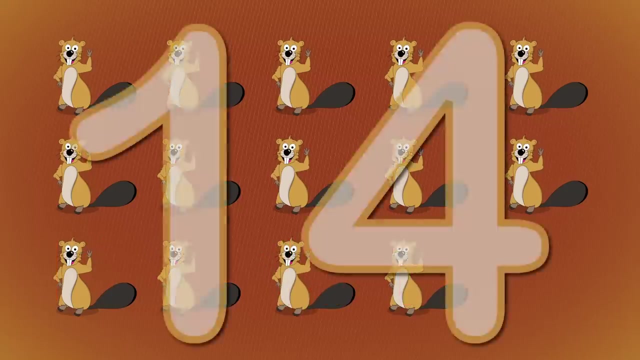 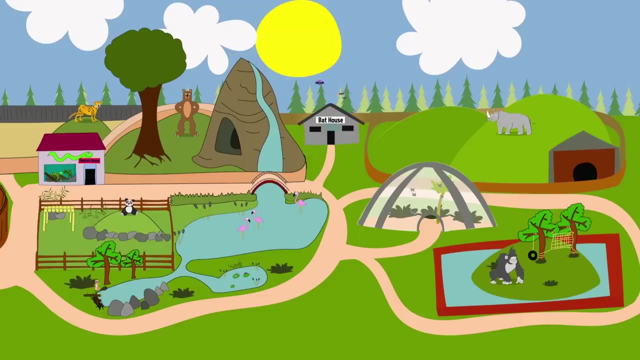 Thirteen cheetahs. Hello, happy beaver, look at your big teeth. Are you building a dam? One, two, three, four, five, six, seven, eight, nine, ten, eleven, twelve, thirteen, Fourteen, Fourteen beavers. 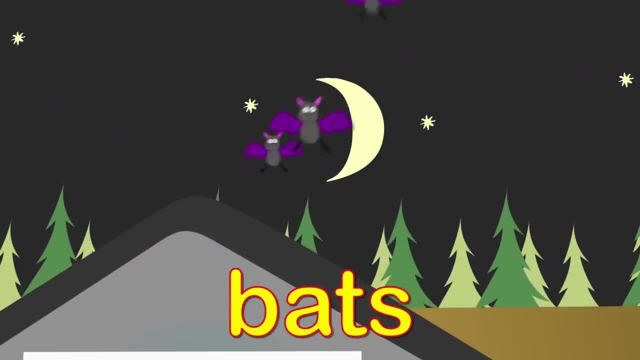 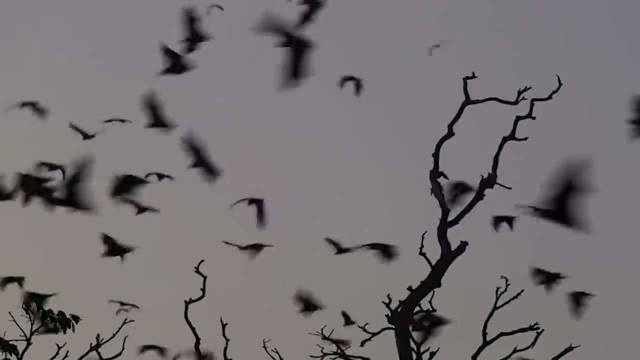 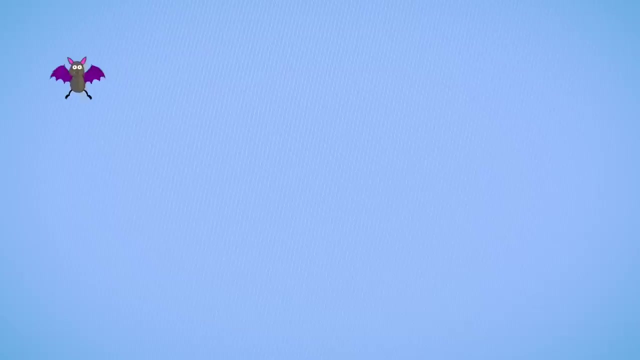 Hello, flappy bats. when it gets dark, the bats come out to play. One, two, three, four, five, six, seven, eight, nine, ten, eleven, twelve, thirteen, Fourteen, Fourteen beavers: One, two, three, four, five, six, seven, eight, nine, ten, eleven, twelve thirteen. 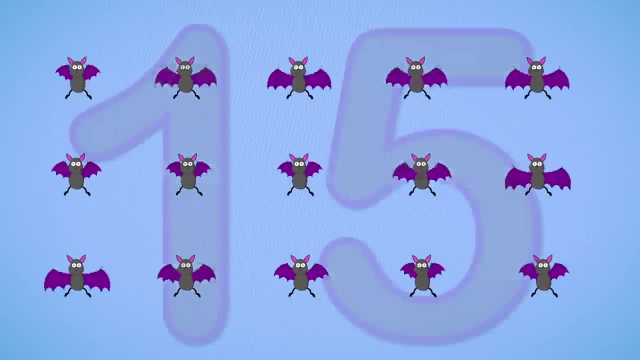 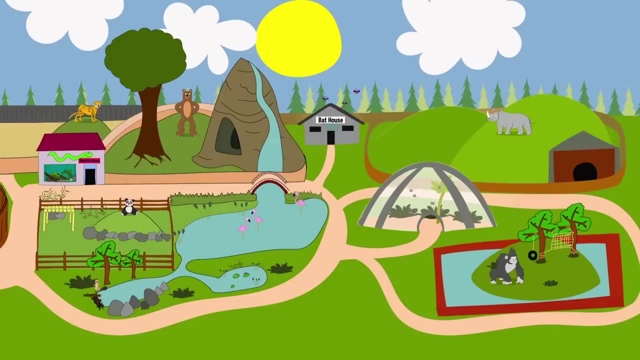 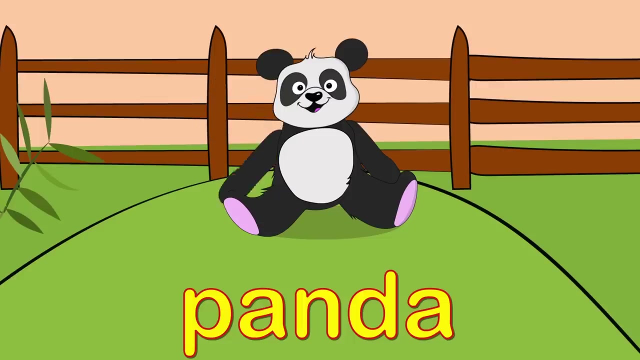 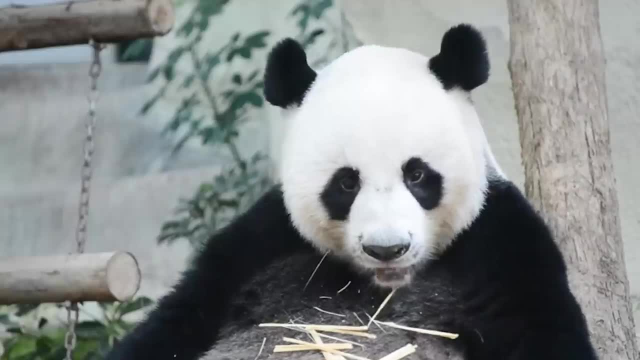 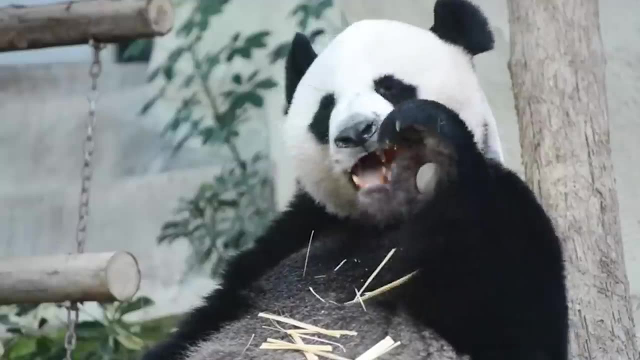 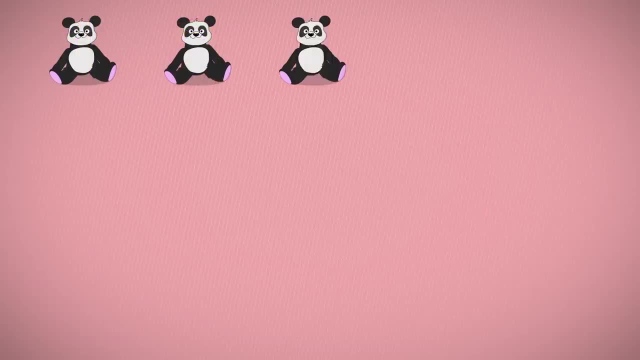 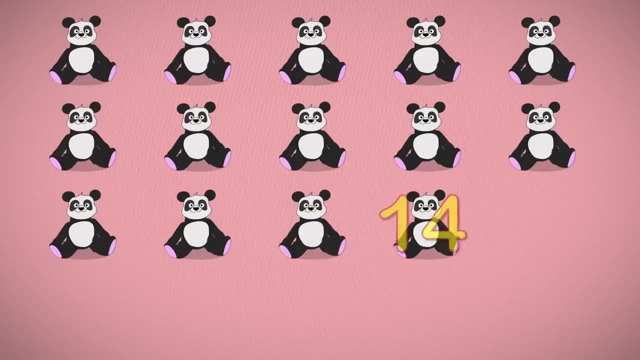 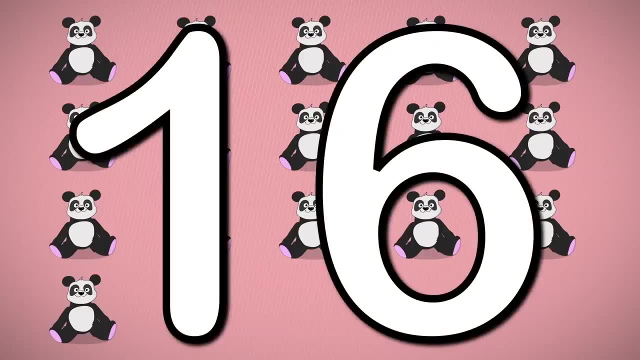 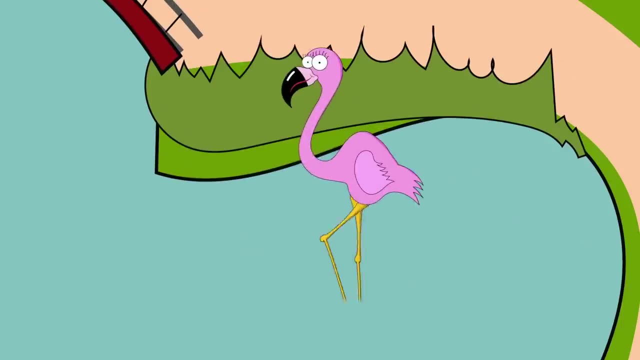 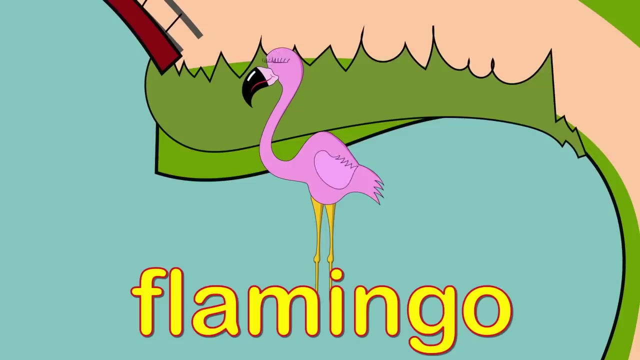 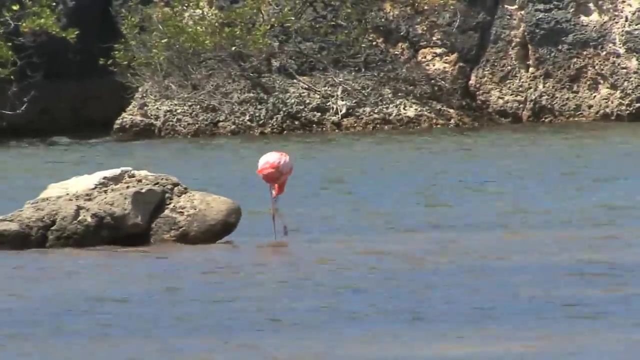 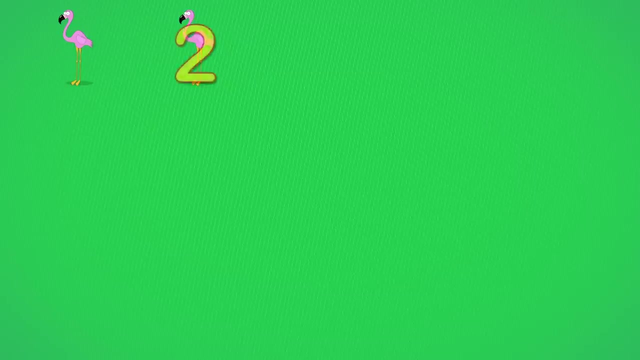 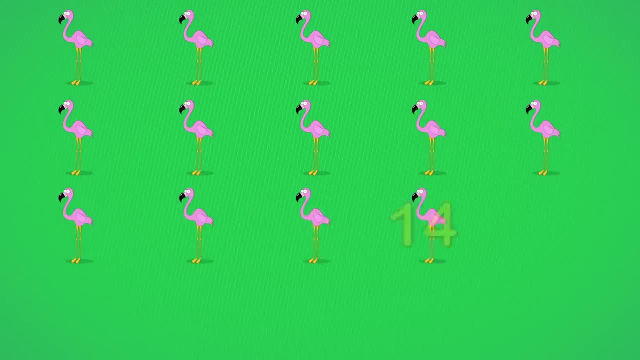 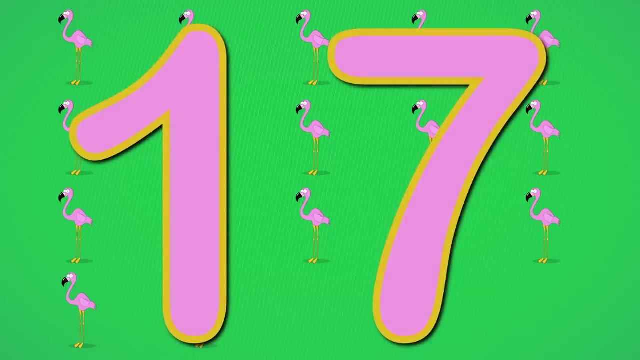 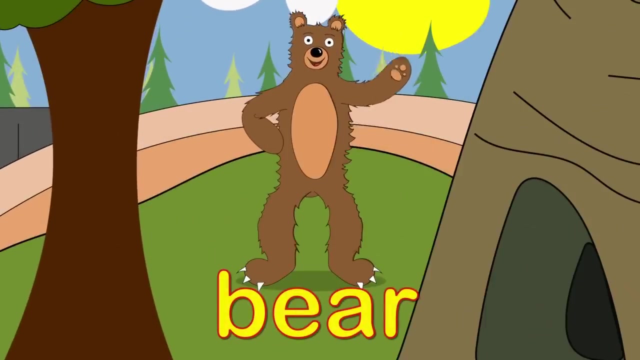 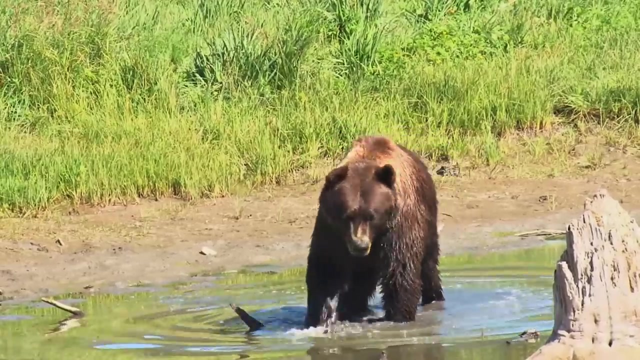 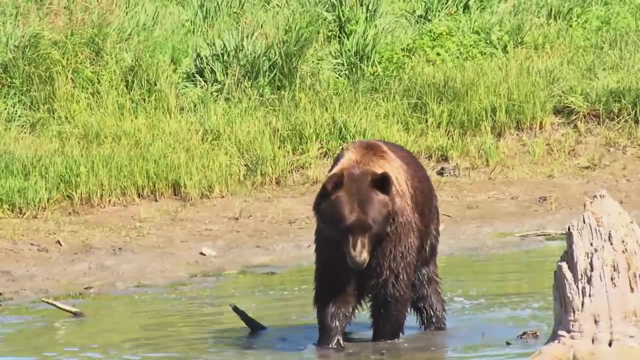 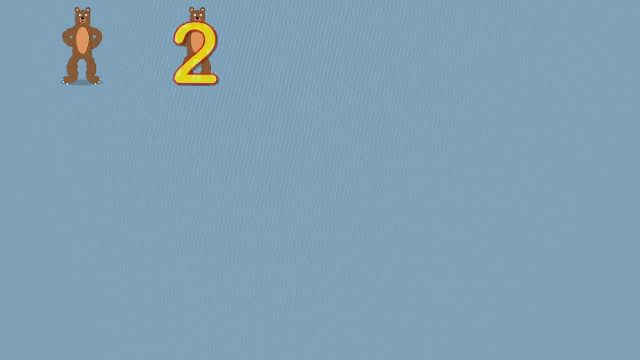 12,, 13,, 14,, 15,, 16,, 17, 17 flamingos Eek. Hello, big brown bear, Star-fingered someplace. Yes, 1., 2., 3., 4., 5.. 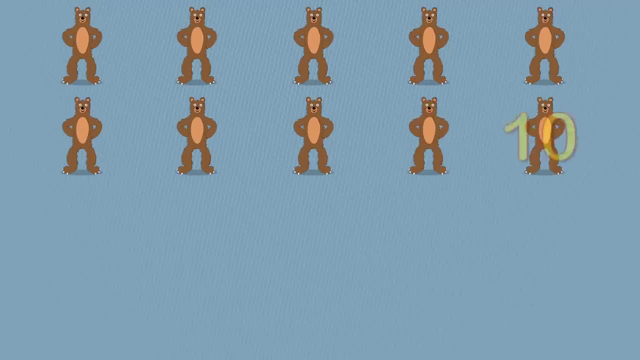 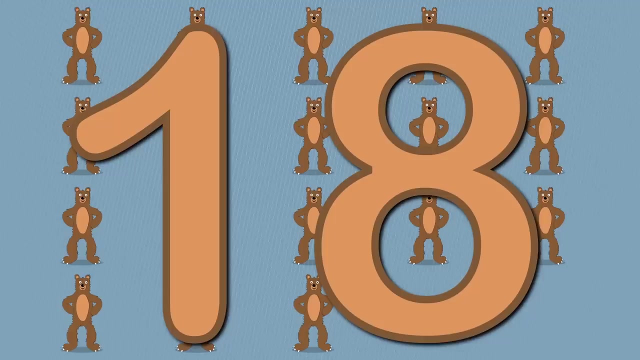 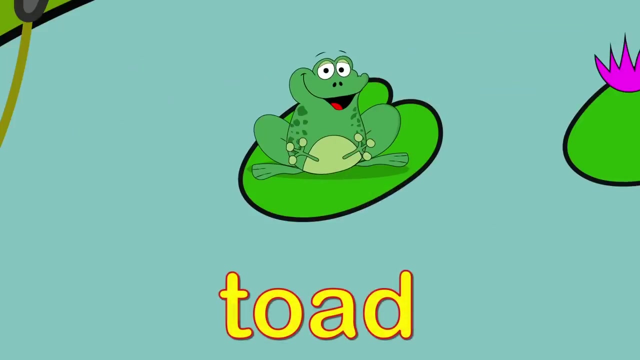 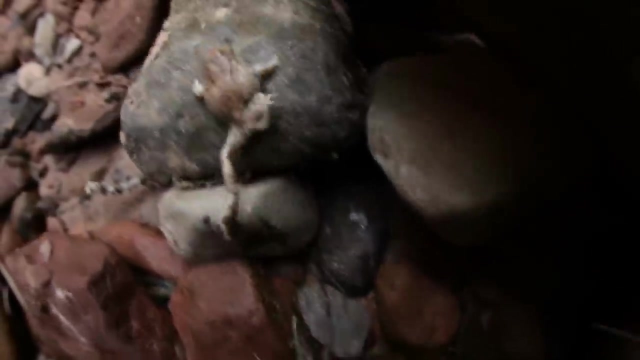 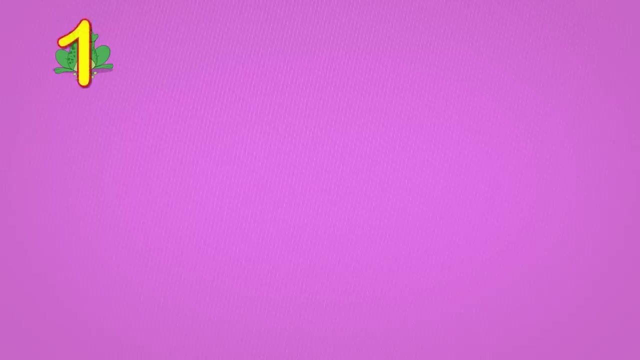 6., 7., 8., 9., 10., 11. 15.. twelve, thirteen, fourteen, fifteen, sixteen, seventeen, eighteen, Eighteen brown bears. Hello, Toad, was that a yummy fly. One, two, three, four, five, six, seven, eight, nine, ten, eleven, twelve, thirteen, fourteen. 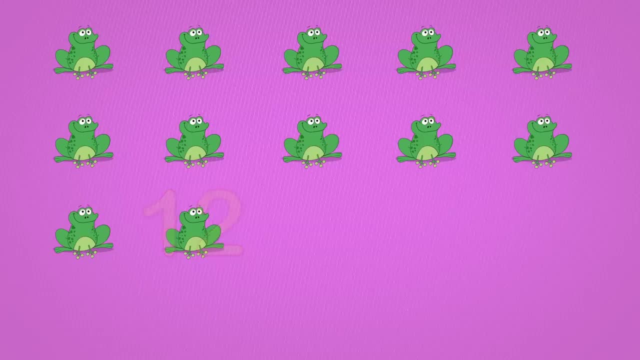 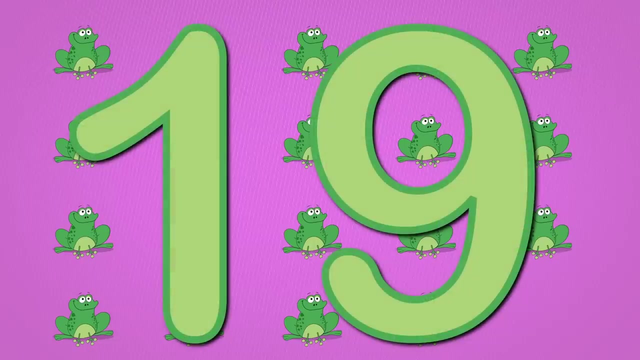 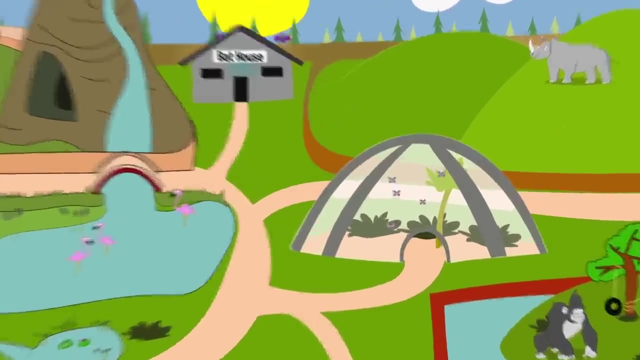 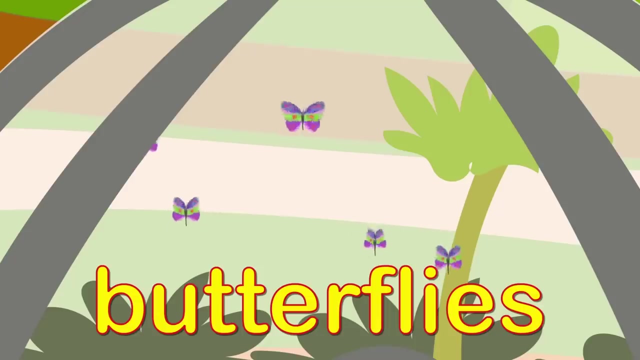 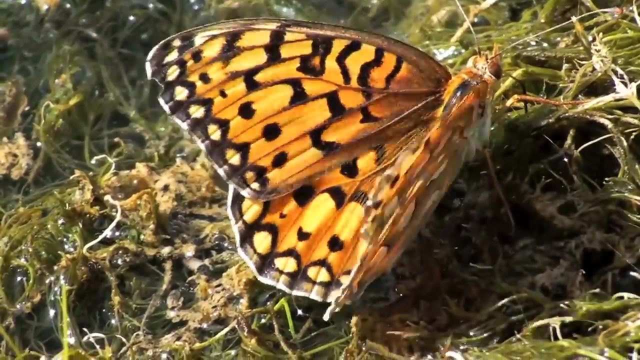 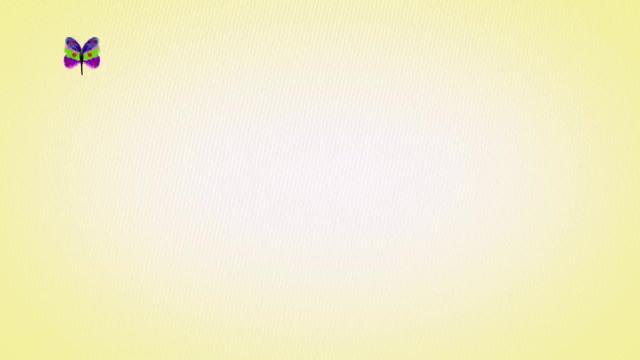 fifteen, sixteen, seventeen, eighteen, nineteen, Nineteen toads. There's only one more new animal to visit. What could it be? Beautiful butterflies, Hello, What can I do for you? One, two, three, four, five, six, seven, eight, nine, ten, eleven, thirteen, eighteen. 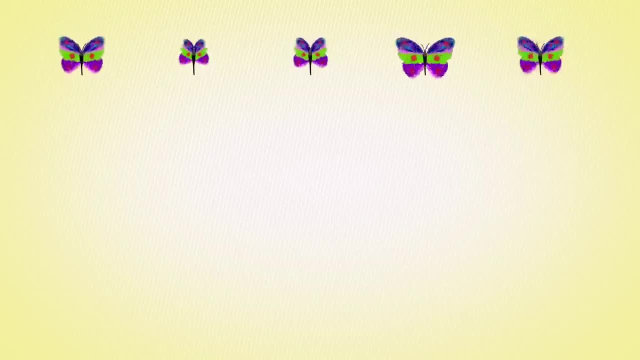 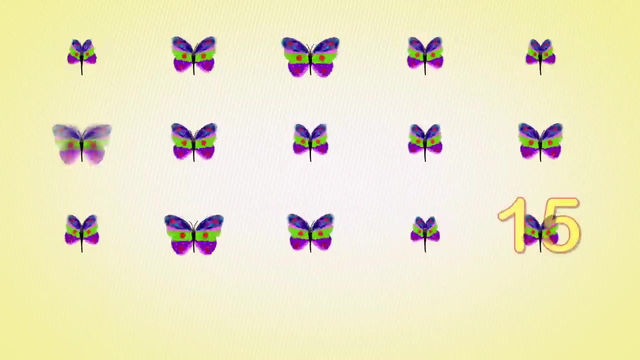 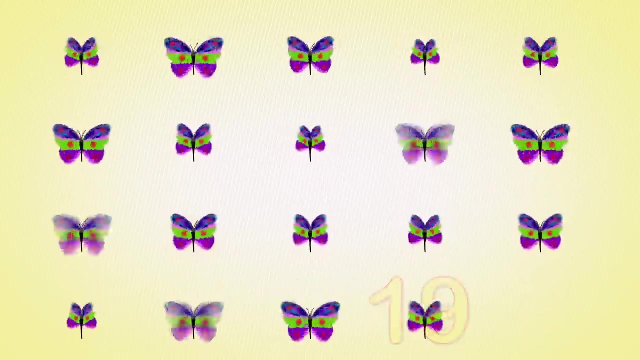 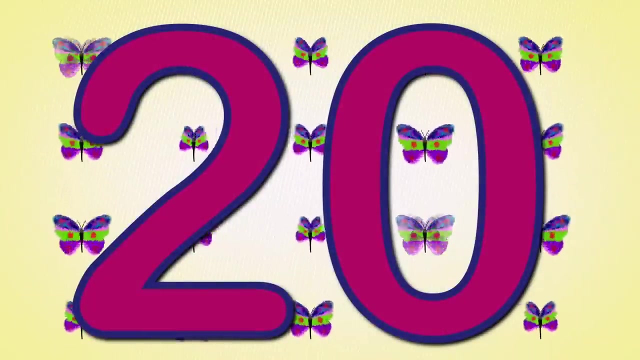 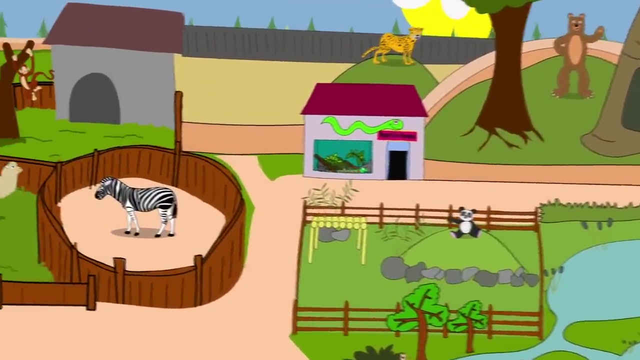 nineteen, twenties, thirteen, eighteen, nineteen. What can I do for you? One Twelve, Thirteen, Fourteen, Fifteen, Sixteen, Seventeen, Eighteen, Nineteen, Twenty, Twenty. Butterflies, Thank you for visiting the animals at Number Zoo today. 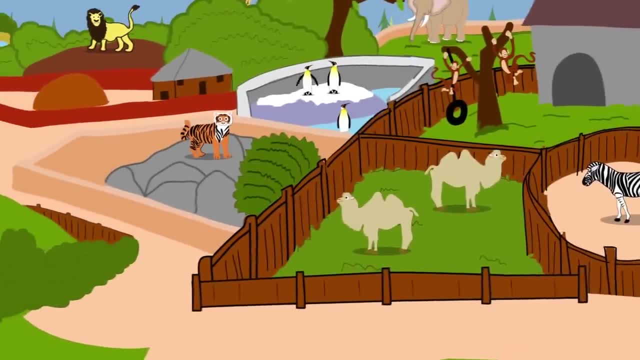 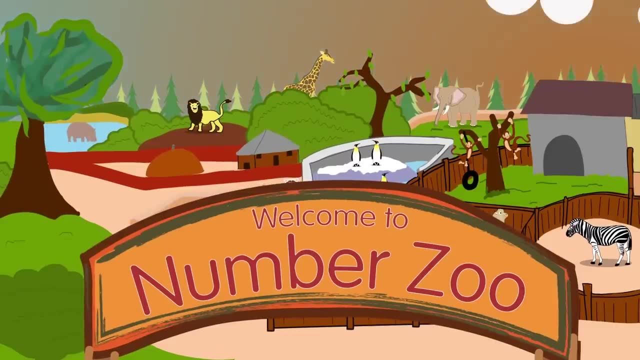 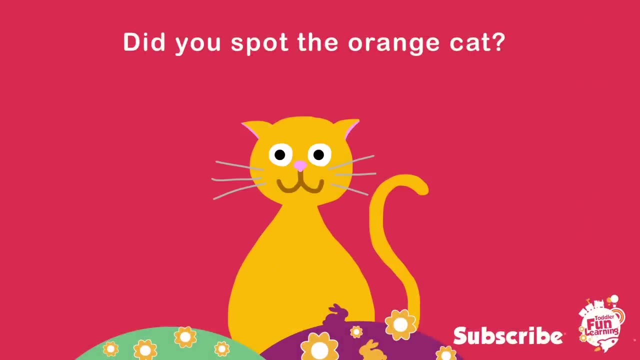 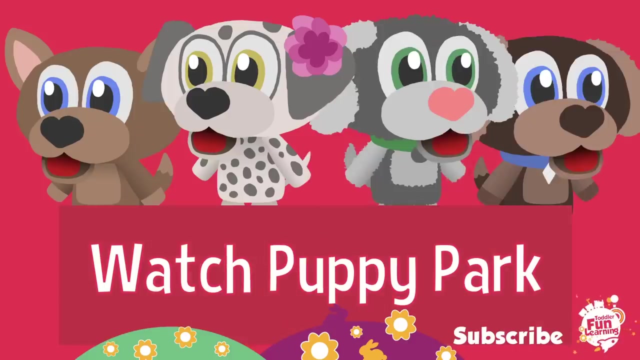 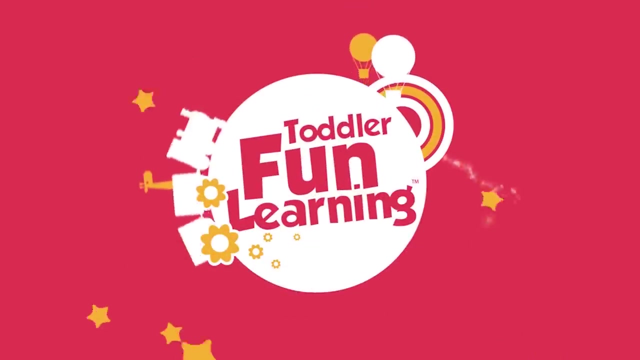 Well done for counting all the way to twenty. See you again soon. Bye, Did you spot the orange cat? Now watch our new series called Puppy Park, And don't forget to subscribe to our channel.